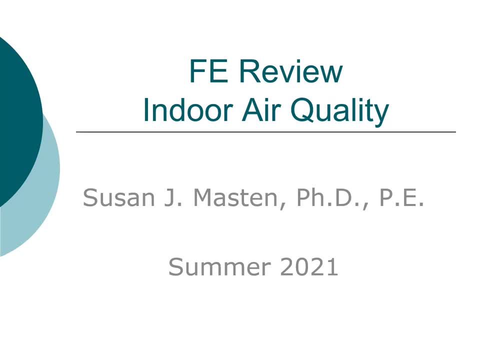 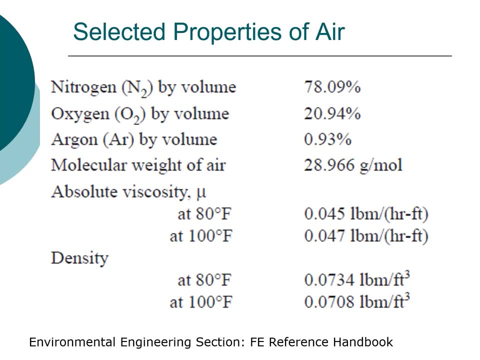 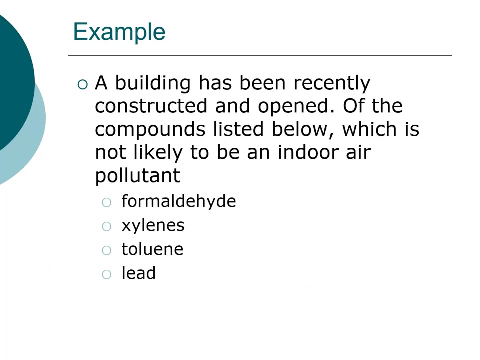 Well, in this EFI review we'll look at indoor air quality. Now again, the section of the EFI reference handbook will somewhat vary, but for this section most of it really is within the environmental engineering section. So a number of the problems that you may very well encounter are based on your knowledge. The answers are not in the reference handbook, so you're going to have to rely on previous course material- what reviews you've done, or just thinking through the problem and using common sense. 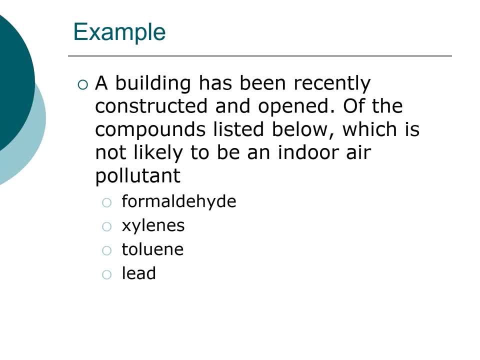 So in this case we have a building that has been recently constructed And opened. Of the compounds listed below you're asked which is not likely to be an indoor air pollutant. So information that's important is that the building was recently constructed and opened. 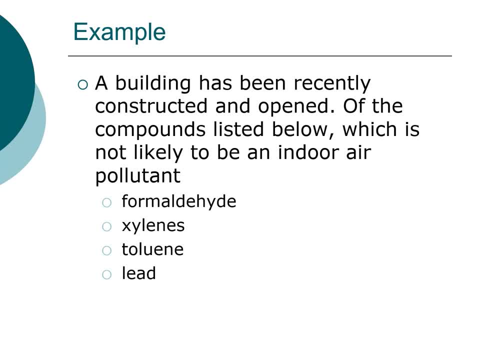 And the choices are formaldehyde, xylenes, toluene and lead. The correct answer is lead And formaldehyde xylenes, toluene- formaldehyde can all be produced from flooring materials, carpeting materials, paints, upholstery. 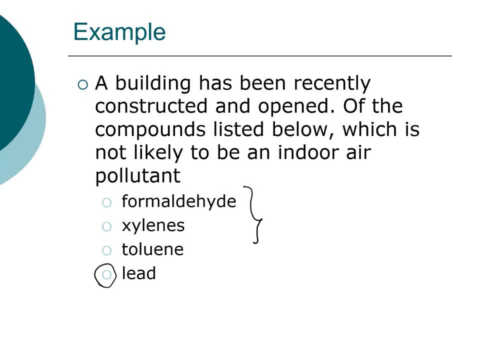 To be released, especially when these are new materials, and it's not unusual to find concentrations in new buildings. In fact, it's referred to as new building syndrome. I. these chemicals Lead. we don't use leaded paint anymore, we don't use leaded gasoline, so it's 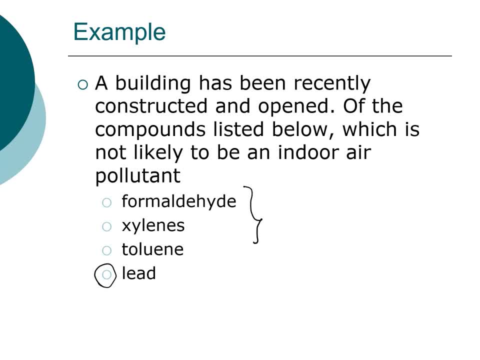 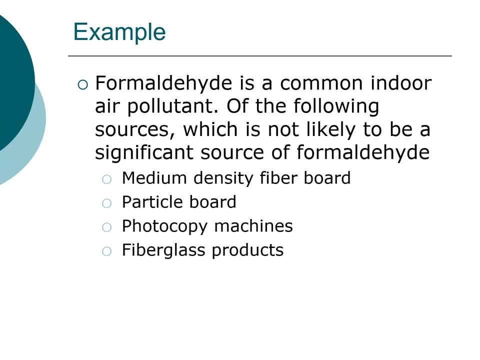 very unlikely that you would find lead in this environment. So in this question here again it's one of these general recall type questions and you're told that formaldehyde is a common indoor air pollutant and you're asked of the following sources, which is not likely to be a significant 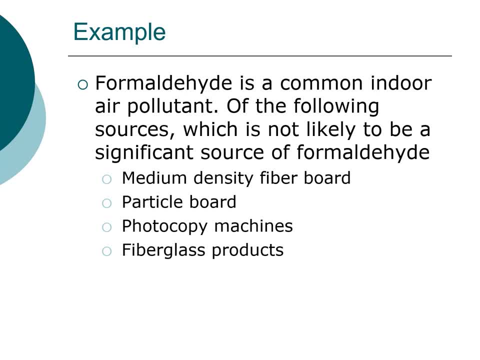 source of formaldehyde And the choices that you're given are medium density fiberboard, particle board, photocopy machines and fiberglass machines. The answer is photocopy machines. Photocopy machines release ozone. the others all release formaldehyde. So in this question here, 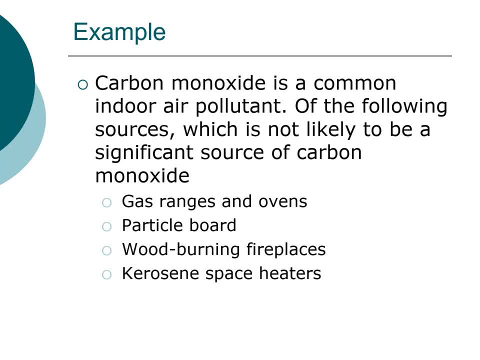 Again, another recall-type question. You're told carbon monoxide is a common indoor air pollutant of the following sources, which is not likely to be a significant source of carbon monoxide. Important thing to remember here is that carbon monoxide is released by incomplete combustion, so it's a product of combustion. 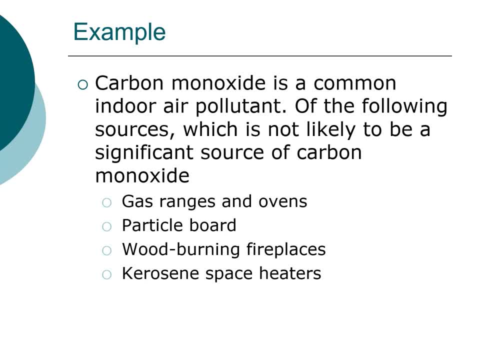 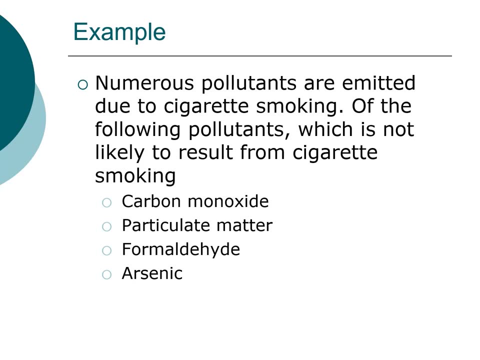 So, if you look, gas ranges ovens involve combustion, wood-burning fireplaces involve combustion, as do kerosene space heaters. So the answer is particle board And the last of these types of questions we have. numerous pollutants are emitted due to cigarette smoke. 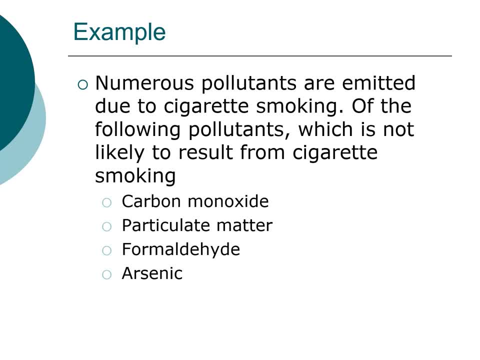 and of the following pollutants, which is not likely to result from cigarette smoking. We just talked about that. carbon monoxide is released from combustion processes. Cigarette smoking is a combustion process, so carbon monoxide is released, as is particulate matter and also formaldehyde. 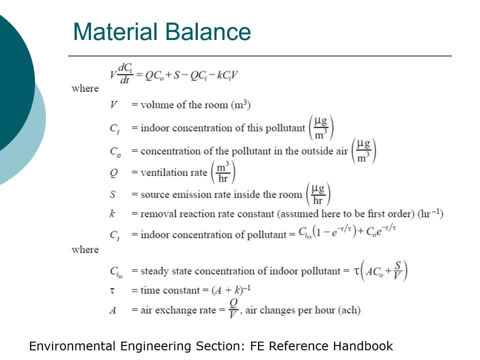 The correct answer is arsenic. So the next set of problems we'll look at pertain to mass balance or pertain to computational-type problems. really, mostly, they do stem from a mass balance approach. The first equation that we'll look at is from the environmental engineering section. 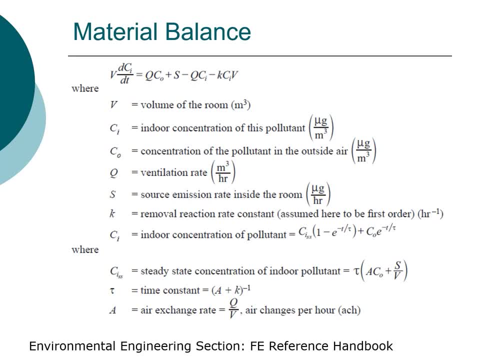 In fact, all of the equations that we'll look at in this unit are from the FE Reference Handbook, Environmental Engineering section. So we have looked at mass balance throughout a number of your courses. You've started in E and E-280,. you've looked at those in E and E-489, E-483.. 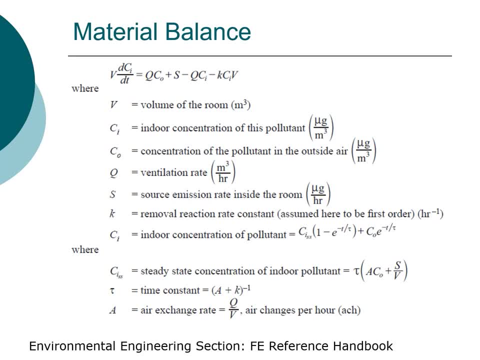 Approach is identical. A couple of things to remember here. Okay, this is written as V DC DT. Remember we've taken volume out of the differential, so we've assumed that we have constant volume And that first term QC-naught. 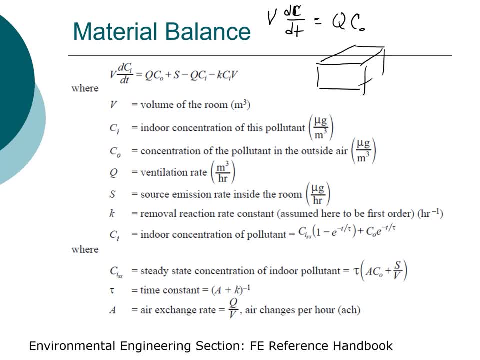 that is the term for the input of your contaminant of interest from the outside. So we have a flow in and in this case, C-naught is the concentration of the pollutant in the outside air. We have a source term inside. 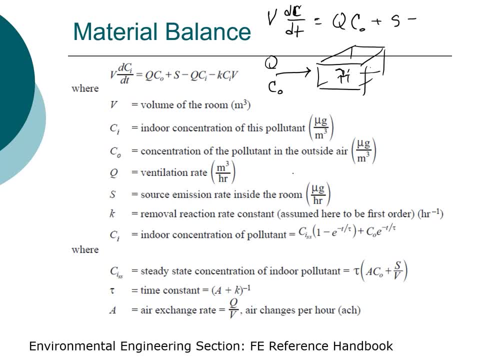 And we have a term for the pollutant leaving. so Q-in equals Q-out, so we'll just use Q And this problem uses C, sub I, or the indoor concentration of the pollutant. So let's note the nomenclature is a little different from what we've used. 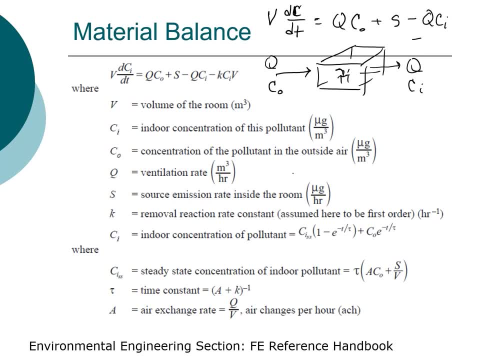 in courses, and then the last term describes first order decay. so we've used kcv. so k is the first order decay. constant c sub i, the concentration in the system, and v is the volume. we've also know in here we've assumed that the concentration leaving is equal to the concentration at any point. 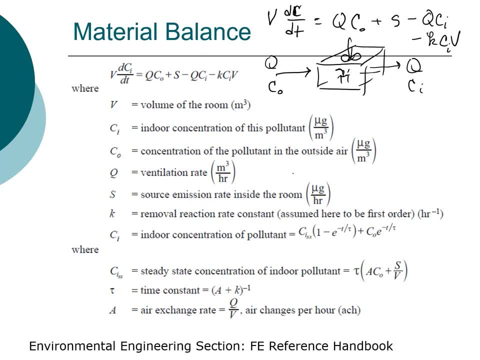 in the system, so we've also assumed that we have a completely mixed system. now the equations that they're giving you here are a little bit different in formulation. they use the term tau, the time constant, and note that that is only the期 MITU time constant. 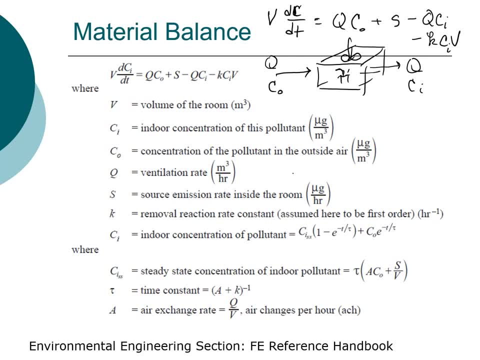 just A plus K, and A is the air changes per hour. so the air exchange rate K is your decay constant. make sure your units are consistent. And then the steady state concentration note is written in terms of tau: the air exchange rate, your concentration entering the system, plus the source term divided by volume. 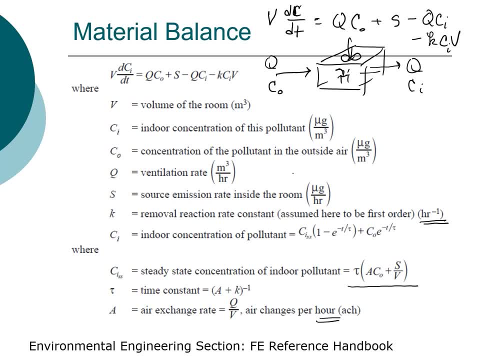 It's identical to what we've done in our classes. it's just a slightly different formulation. Same thing here, slightly different formulation from what we have done in class. The one thing to note with this Is that it's assuming. this formulation here assumes that the concentration at time zero. 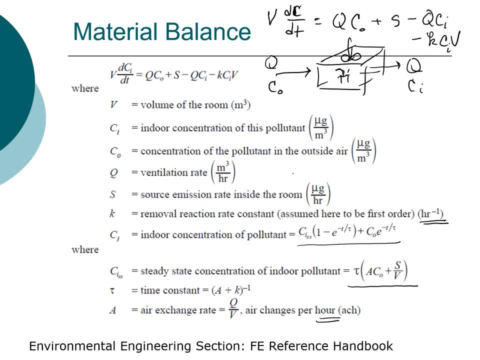 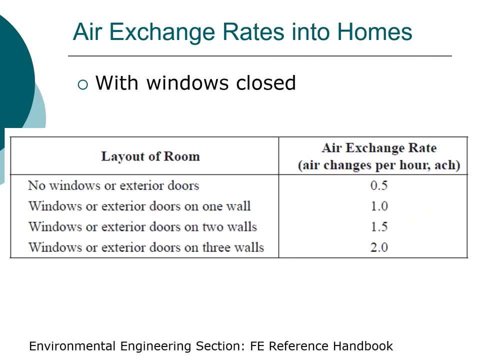 is equal to the outside concentration. so that's an important caveat in this formulation here. And then it also provides you with some information about the air exchange rates into homes, so it gives you various different conditions of the room and how that moves. So that gives you a little bit more detail. 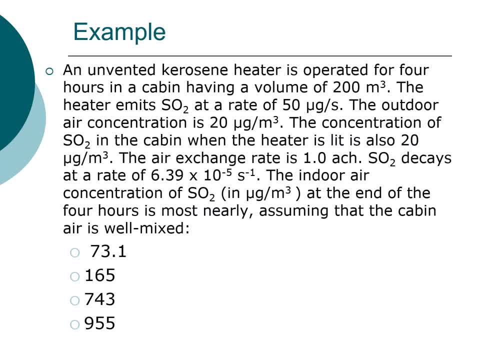 So let's do a first problem here. We have a situation where we have an an-vented kerosene heater and it's operated for four hours in a cabin and you're told that the volume of the cabin is 200 cubic meters. 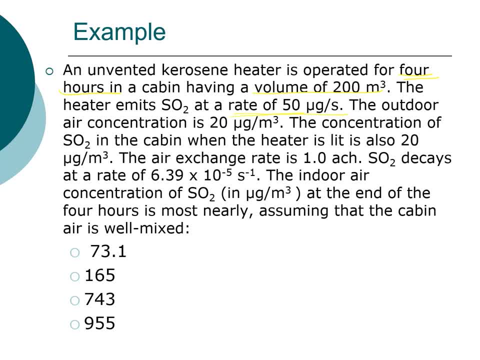 The heater emits SO2 at a rate of 50 micrograms per second, So that's a significant difference. All right, So we've just written this down, So let's look at the solution. The outdoor air concentration is 20 micrograms per cubic meter. 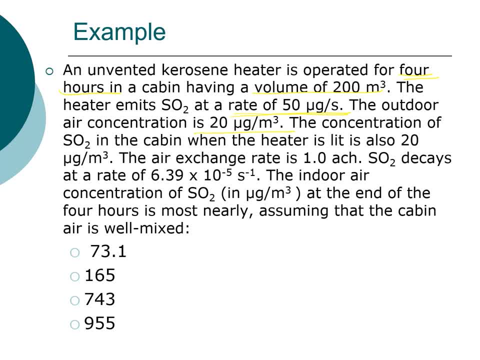 and the concentration in the cabin when the heater is lit is also 20 micrograms. So that's what I just mentioned, that we're assuming that initial concentration is the same as the outdoor air concentration. You're told that the air exchange rate is one air change per hour. 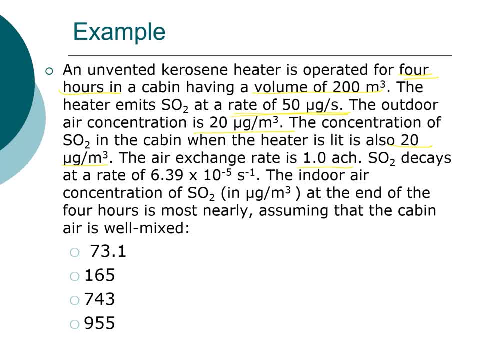 You could, in one of these problems, have been told something about the configuration in the room, in which case you'd have to look up the air exchange rate And you're given a decay rate for SO2, and you are asked for the indoor air concentration at the end of four hours. 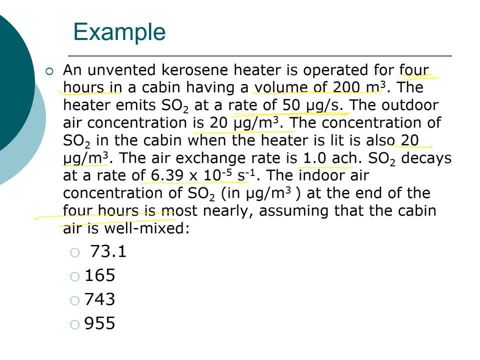 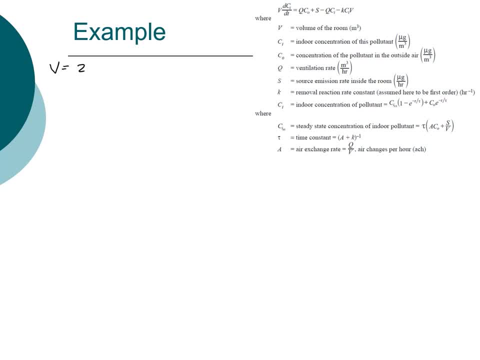 We're going to assume, as we just discussed, that the cabin is well lit, So let's look at this problem. We'll write down the parameters We have. volume is equal to 200.. Cubic meters. Their source term is 50 micrograms per second. 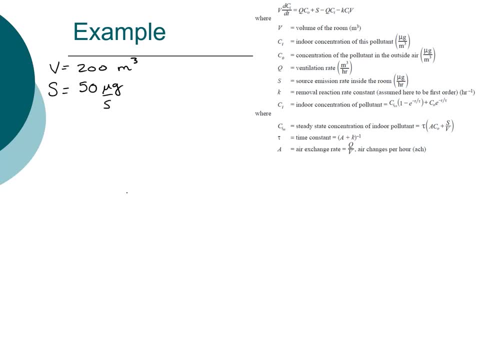 We want that in mass per hours. So if we multiply that by 60 seconds per minute and 60 minutes per hour, then that is equal to 18,000 micrograms per C0.. Concentration in the outdoor air, we're told, is 20 micrograms per cubic meter. 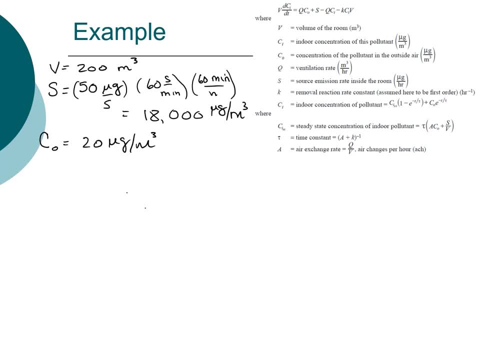 And we've said that that is the concentration when the heater is lit. You're told that the air exchange rate is one air change per hour. You're given a decay constant in inverse seconds. Again, we want that in inverse hours. So we'll multiply by 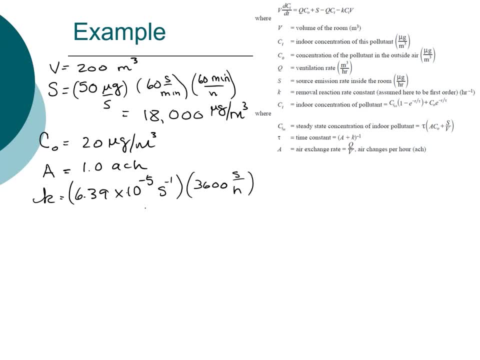 3,600 seconds per hour, and that is equal to 0.23 inverse hours. The first calculation we need to do is to determine tau, and that is equal to a plus k minus 1. So that is equal to 1.0 plus 0.23. 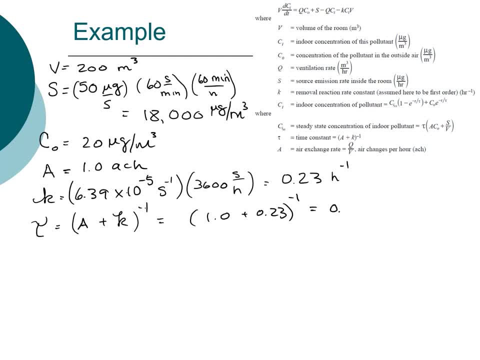 Take an inverse of that sum And that is equal to 0.23.. 813 hours And we'll calculate the indoor air concentration at steady state, And this is because of the way that the equations are given here. And that is equal to tau ac0 plus s over v. 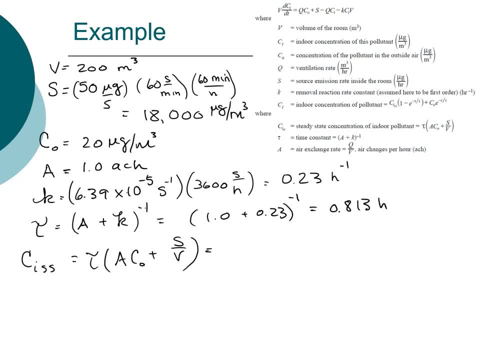 You could derive this based on what we've done in class, but since you've given that you're done, So we're going to calculate the tau ac0 plus s over v, And we're going to calculate the tau ac0 plus s over v. 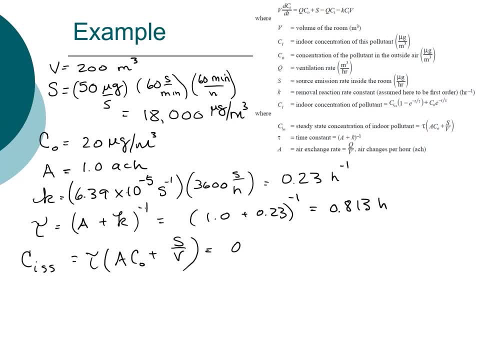 So we're going to calculate the tau ac0 plus s over v. you've given this equation, we use that and that is equal to 0.813 hours times a, 1.0 inverse hour times c, naught, which is 20 micrograms per cubic meter, plus s, which is 18 000 micrograms. 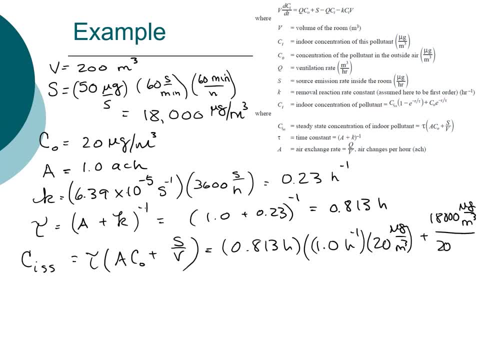 per cubic meter divided by the volume, which is 200 cubic meters, and we need to close those parentheses, and that is equal to 747 micrograms per cubic meter. and then you give an equation for ct, so the concentration at time, t, and that is equal to. 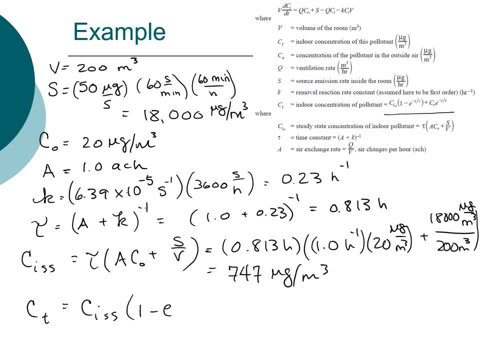 c iss 1 minus e to the minus t over tau, plus c 0 e to the minus t over tau, and that is equal to 747 micrograms per cubic meter times 1 minus e to the minus 4 over tau, which is 0.813. 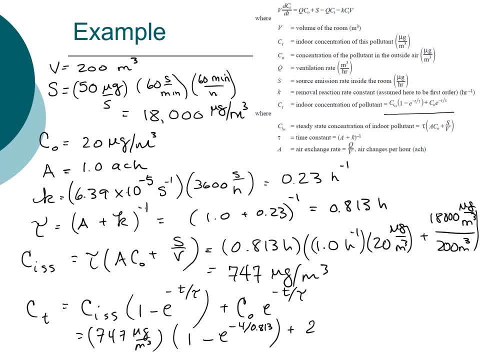 plus c sub 0, that's the 20 micrograms per cubic meter times e to the minus 4 over 0.813, and that is equal to 743 micrograms per cubic meter. so that is the correct answer. I'm just going to stick it in. 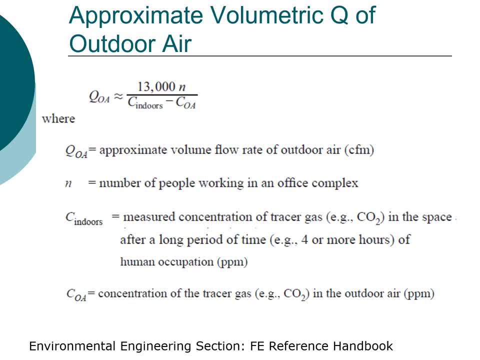 I don't have to caring about it several times because they all get the answer for this problem, And so I'm just going to write the answer for this problem In this next problem here, which is actually taken from the industrial hygiene literature. it's an attempt to determine the relationship between number of people working in an office. 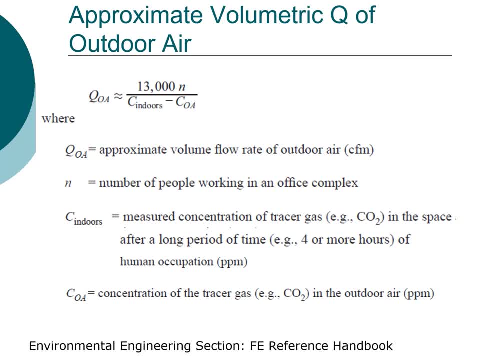 complex the concentration in this indoor space and then the concentration in an indoor space after a long period of clogging, after a long period of time of human occupation. so, for instance, it could be it's just people are leaving for lunch, it could be at the end of the day, and the concentration 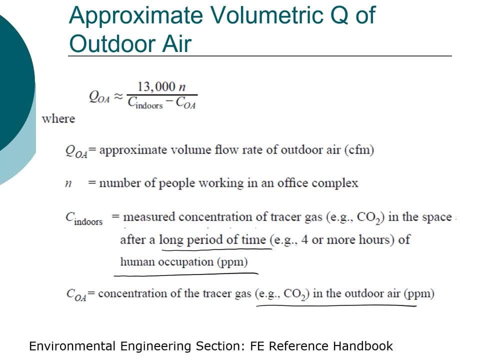 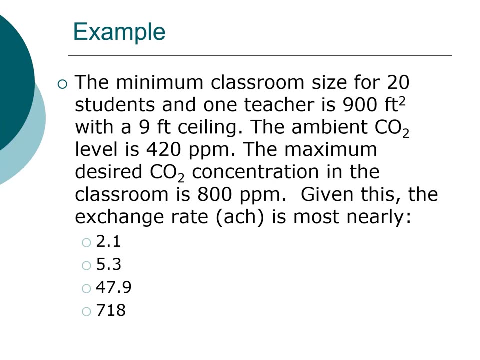 in the outdoor air, and what we can determine from this is an approximate flow rate of outdoor air. so let's look at this next problem and in this case, here you're told that the minimum classroom size for 20 students and one teacher is 900 square feet with a nine foot ceiling. 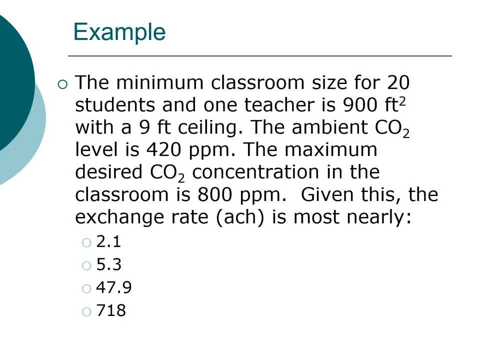 the ambient co2 level is 420 parts per million. the maximum desired co2 concentration in the classroom is 800 parts per million. that's 420.. could even say that it should be lower than that, but at 800 you start to see children get sleepy. 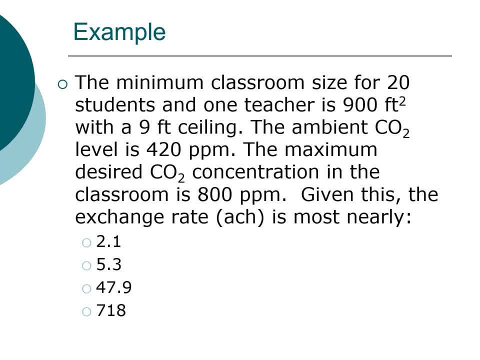 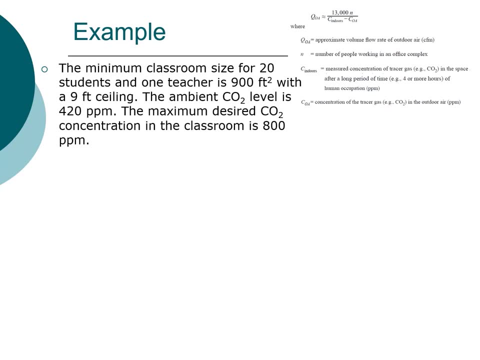 lack of focus. so we want to make sure that we keep that concentration, less than 800, and given that the required air exchange rate is most nearly, and you're given a number of choices, so let's look at this problem here. so, again, using their notation c, sub o, a or the f. 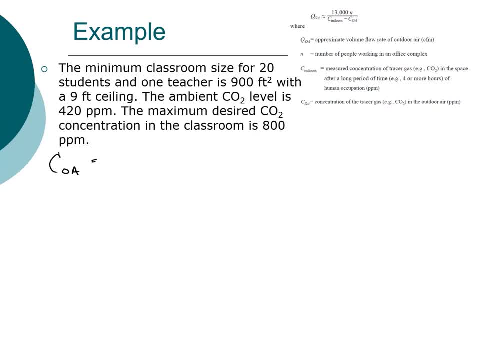 concentration of co2- and we're using co2 as a tracer gas- is 420 parts per million c indoors, so that maximum concentration that we desire is 800 parts per million. n is equal to 21. we have 20 children, students, plus one teacher, and then it's just. we can calculate q. 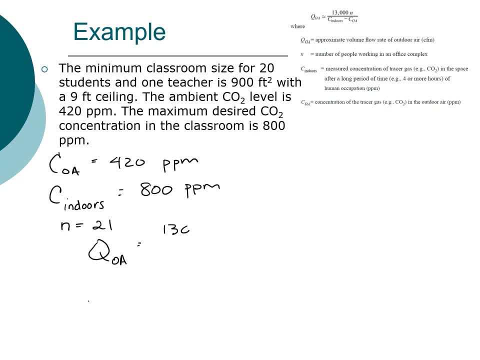 o, a. a is equal to 13 000 times n, so that's 21 students that we have divided by 800 minus 420, and that is equal to 718 cubic feet per minute. and just note the units here. so the way that this is written. 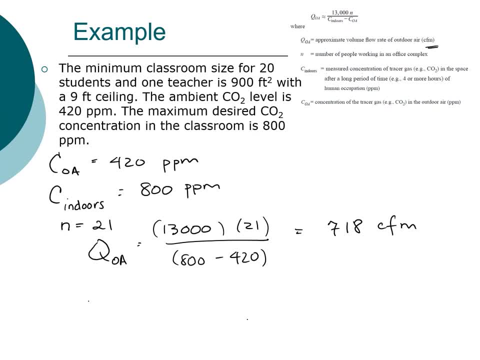 is your answer. your flow, volumetric flow rate is in cubic feet per minute. you were asked for air changes per hour, so a is equal to 718 feet cubed per minute. there are 60 minutes in an hour and we will divide this by the area, so we have 900 feet squared times the height of nine feet. 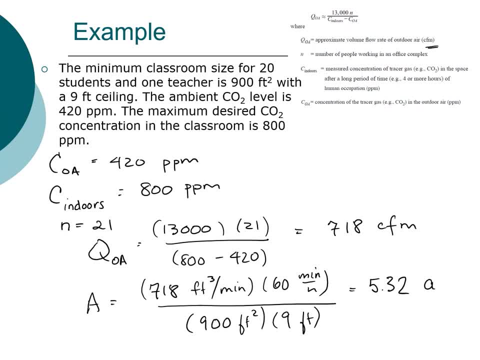 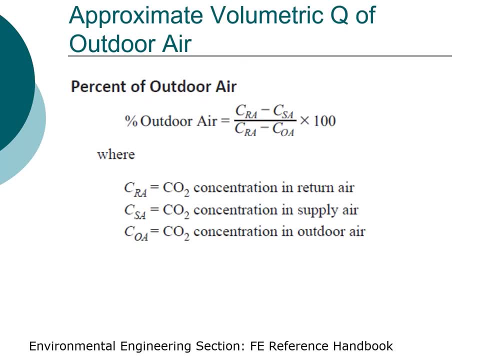 and that is 5.32 air changes per hour. so that is the correct answer here. this next equation actually comes from ASHRAE, and ASHRAE is the American Society of Heating, Refrigerating and Air Conditioning Engineers Incorporated, and they have a standard and it's ASHRAE. 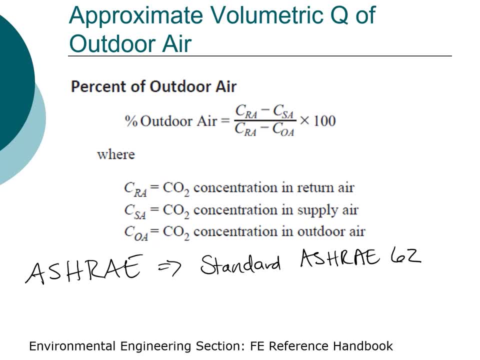 62, which pertains to ventilation levels for air. This is an average of 60 degrees Fahrenheit, one hundred percent of air, one hundred percent of air, One hundred percent of air, one hundred percent. and here's a little bit more information about your air and air temperature. 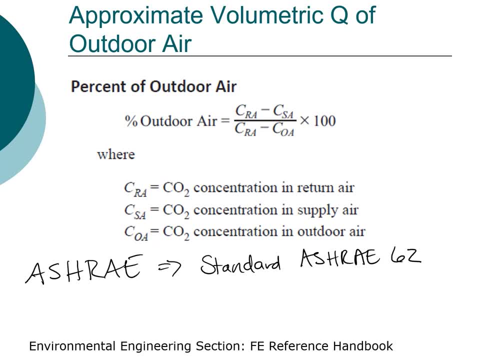 acceptable indoor air quality, and this provides recommendations for the minimum amount of air that is needed per person in defined spaces. so one way that we can calculate the amount of air that we need is with this equation here. so again, CO2 is used as tracer gas. it's easy to measure and we can measure the CO2. 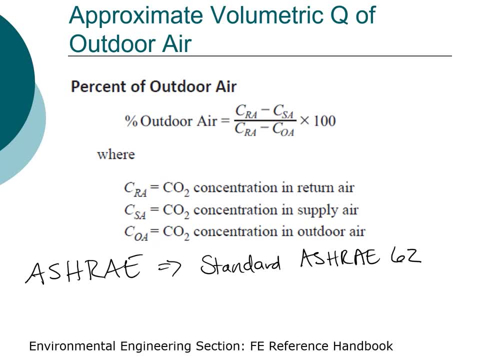 concentration in the return air, in the supply air and the CO2 concentration in the outdoor air. so we're looking at using outdoor air in order to bring in fresh air, to provide a cleaner, refreshed atmosphere. also used to prevent or to reduce potential exposure to any sort of. 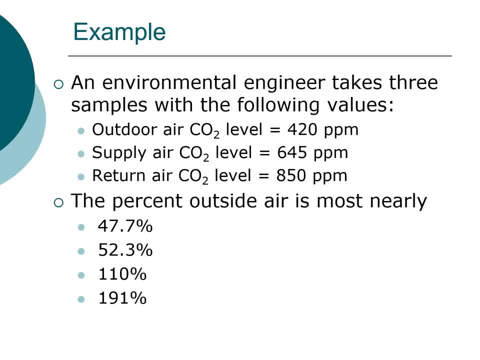 infectious disease. so we have a problem here where you were told that the environmental engineer takes three samples with the following air values. so the outdoor air CO2 level is 420 parts per million. the supply air has only 2 hours, so the temperature is different. that is why we don't need that. 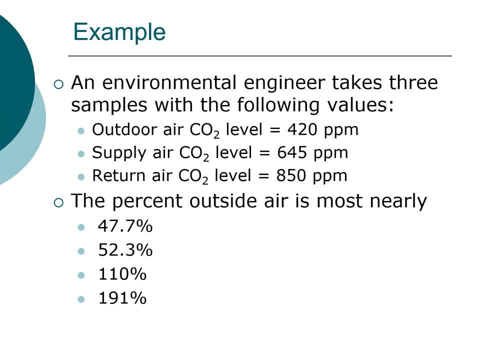 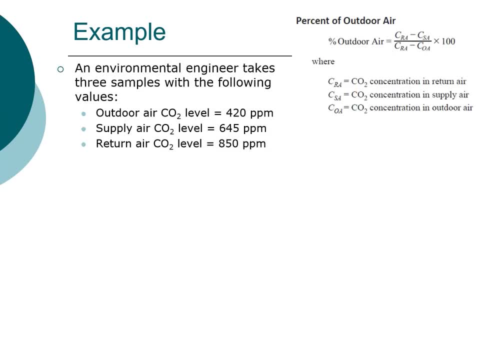 has a CO2 level of 645 parts per million and the return air is 850, and you're given a number of choices again, and then the question is: what percent outdoor air do we need to provide? and the percent outdoor air is just the concentration of the CO2 and the return air. 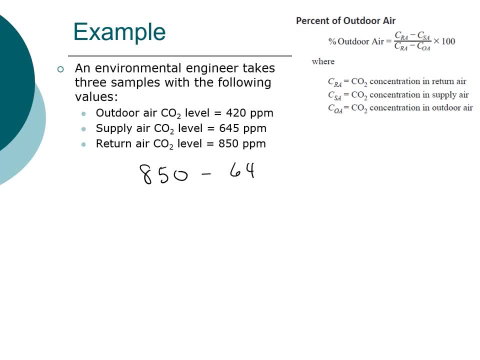 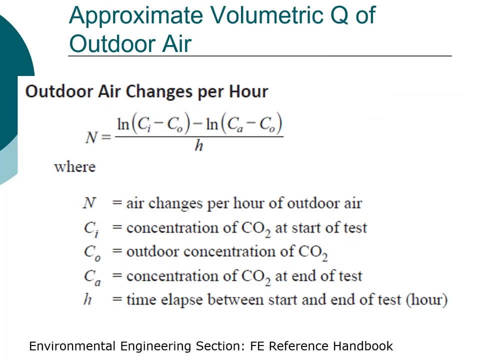 minus the concentration in the supply air, divided by the concentration in the return air, minus the concentration in the outdoor air, and we'll multiply that by 100 to get percent, and that is 47.7 percent. So that is the correct answer there. The final problem that we'll look at. 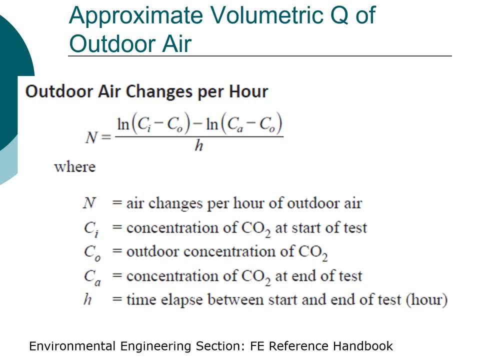 again is from an ASHRAE industrial hygiene test. Again, you're given this equation here, and here we can determine the number of air changes that are required to maintain a certain level of pollutant. In this case we'll look at CO2. so 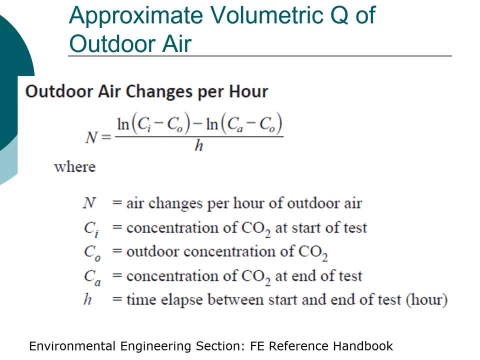 it's based on CO2 levels, again as a tracer cast, and it's also based on an exponential decrease in CO2 levels over time. And what we measure is: we measure the CO2 at the start of the test, we measure the outdoor concentration of CO2 and we measure the concentration of CO2 at the end of the test and the time. 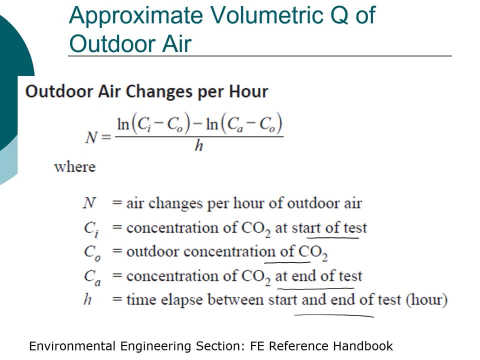 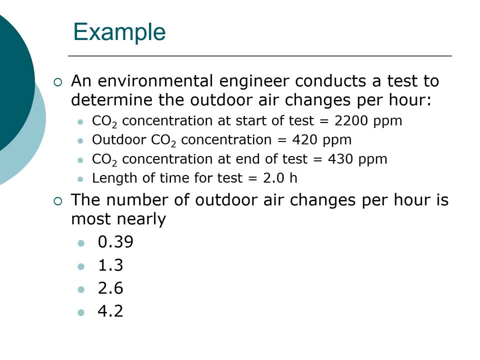 lapse between the start and end of the test. So we have again a set of data that's provided to us. So we have an environmental engineer conducts a test to determine the outdoor air changes. So we have a CO2 level at the start of the test. we have the outdoor CO2 concentration, we have the concentration at the end of the test, which is two hours, and you're asked for the number of outdoor air changes per hour. 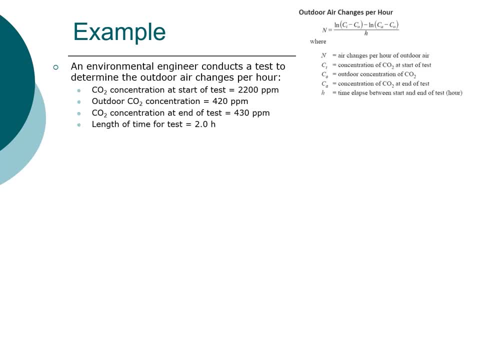 Again you're given a number of choices, So again let's just write this and we'll use their notation. So C sub i is the concentration of CO2 at the start of the test. C0 is the concentration of CO2 from the outdoor air, so it's the concentration outside.